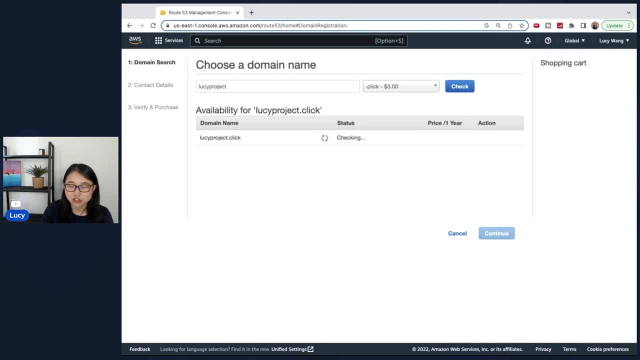 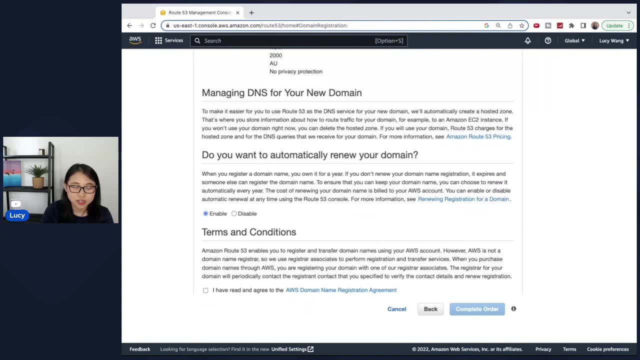 choosing click is because it's the cheapest one I can find. Check if it's available and add it to your cart and fill in your contact details. After I type in my details, the final stage is to accept the terms and conditions. When you're on this page, make sure you click disable. 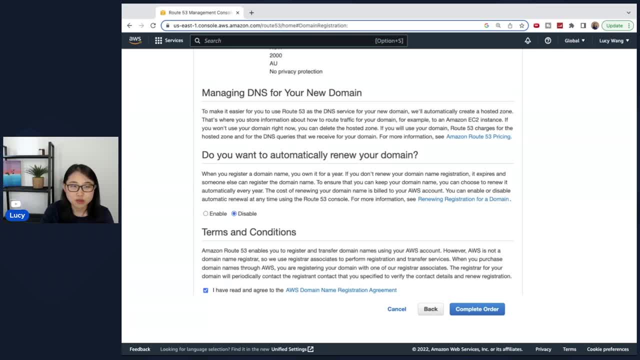 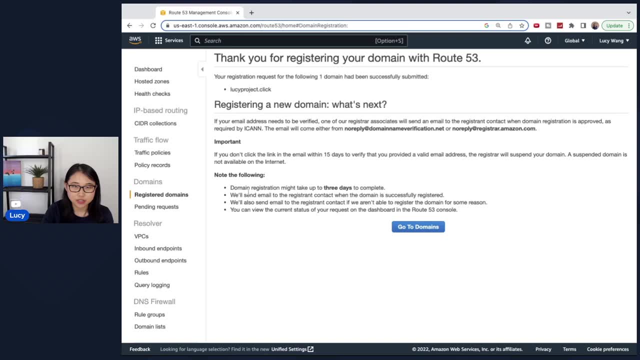 When asked if you want to automatically renew your domain. that way, you won't be charged after one year once your domain expires. Accept the terms and conditions and complete order. Okay, so here. it says that the domain registration might take up to three days to complete, but usually it. 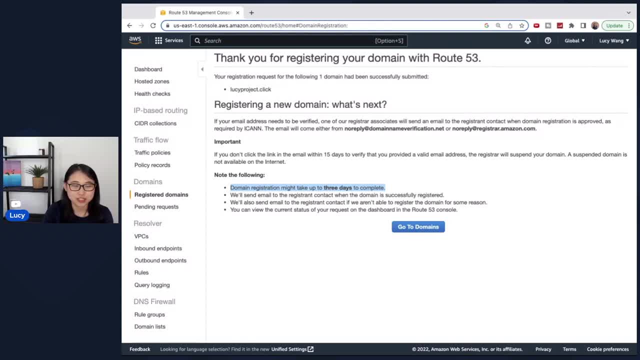 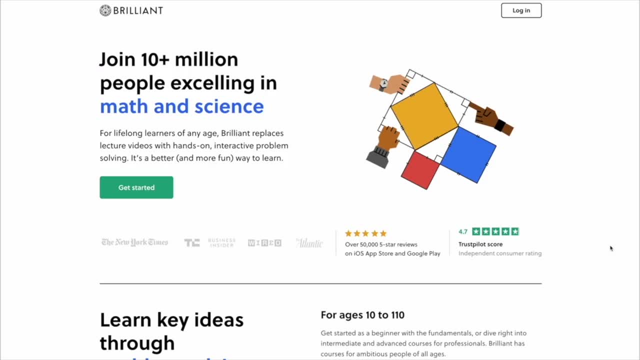 only takes around 10 minutes for me, So while we're waiting for the domain registration to be completed, I'd like to take a moment to tell you about today's video sponsor, Brilliant. One of the best ways to understand technical concepts is by going back to the fundamentals. Brilliant is a 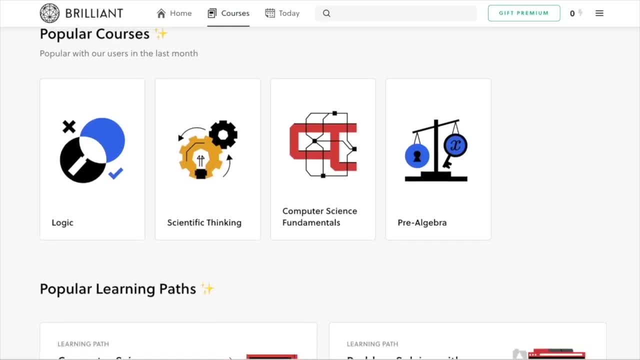 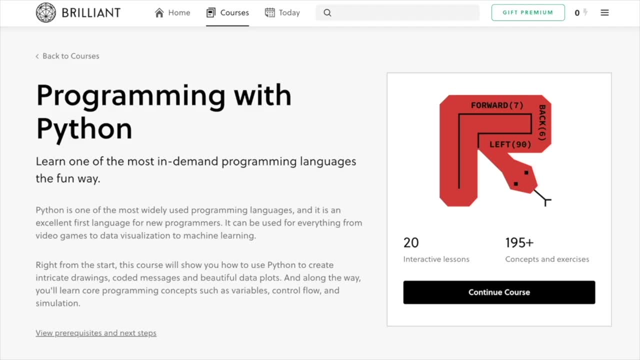 domain that focuses on courses in maths, science and computer science. The lessons are very interactive and you'll be guided through fun problems that come with detailed solutions. If you're someone looking to start your career in the cloud industry and want to improve your programming skills, you can check out their programming with python course You can get. 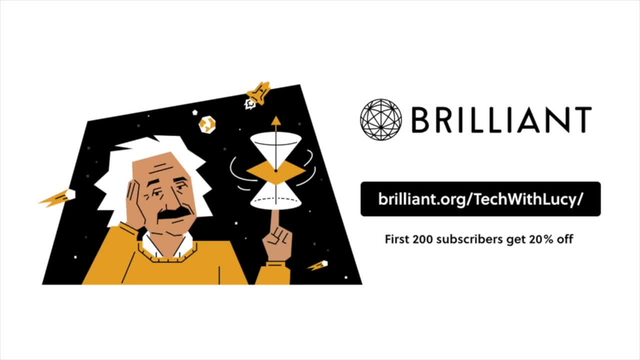 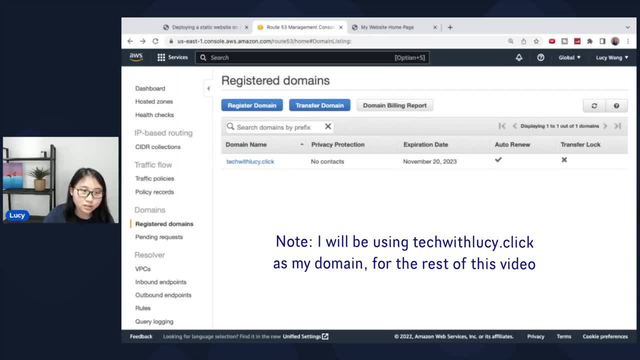 started with Brilliant for free by heading to brilliantorg. forward slash tech with lucy, and the first 200 people also get 20% off their annual membership. Now let's get back to the video. So, once your domain has been registered, you can then head to the next step. 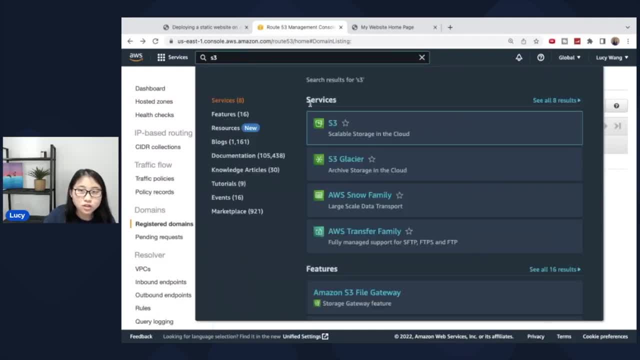 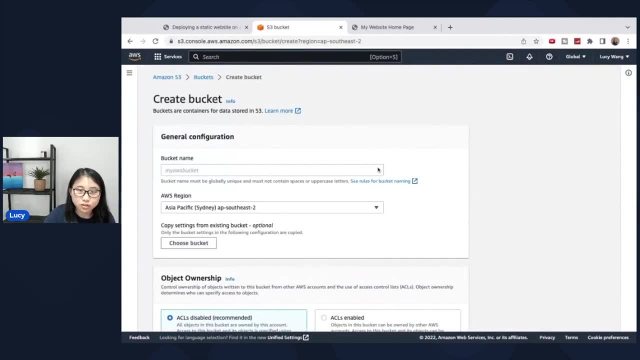 Next step is to go to the amazon s3 page and create a bucket. So this bucket will be used to host our website. So once you click on create bucket, type in the domain name that you registered- tech with lucy dot click. So for this to work, make sure you use the same name as the domain you. 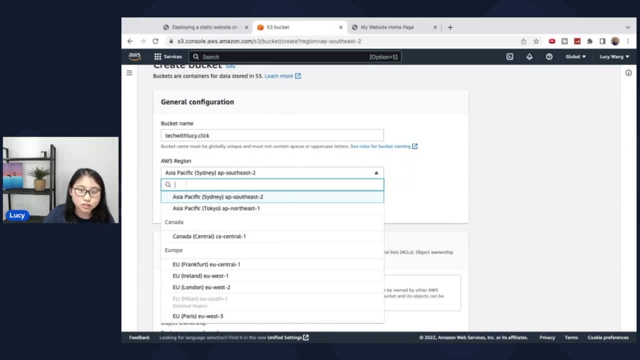 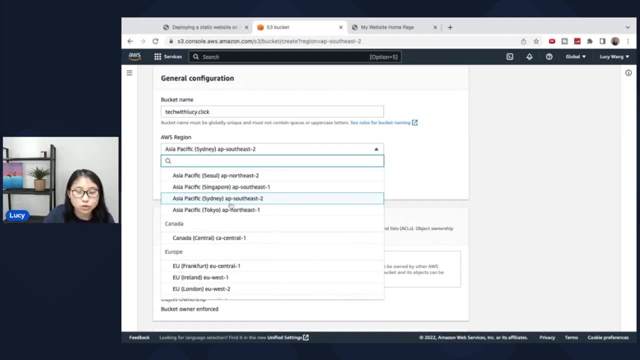 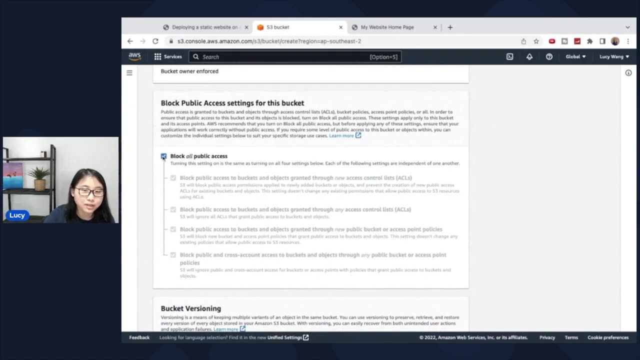 registered For the region. you can select a region that is closest to where you live in order to make sure you have access to your bucket. So in my case, I live in Sydney, so I'm going to select the AP southeast 2 region. Scroll down to the bottom and uncheck this block public access. This is to make 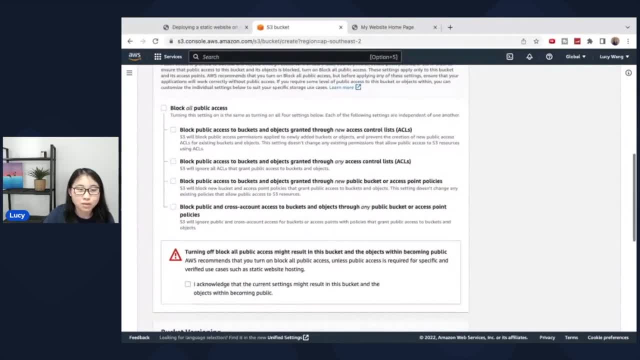 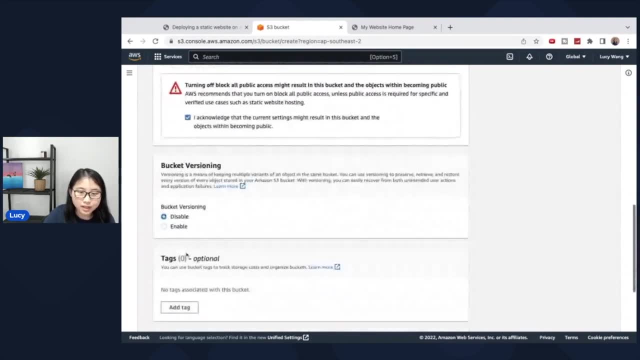 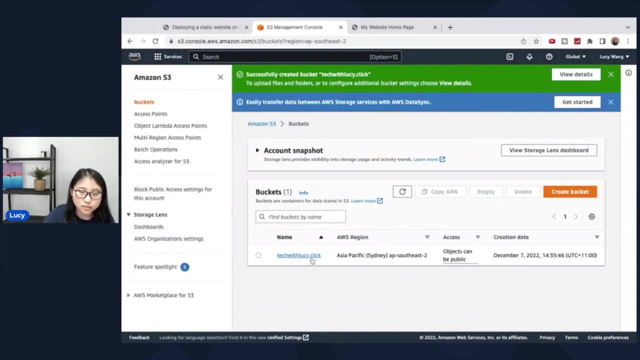 sure that the users will have access to your bucket and make sure it's publicly accessible to others on the internet. Acknowledge this warning and keep all the other settings as default. So once the bucket has been created, you can see here there's tech with lucy dot click. 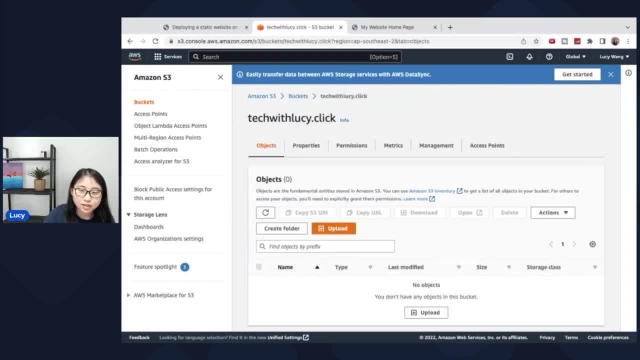 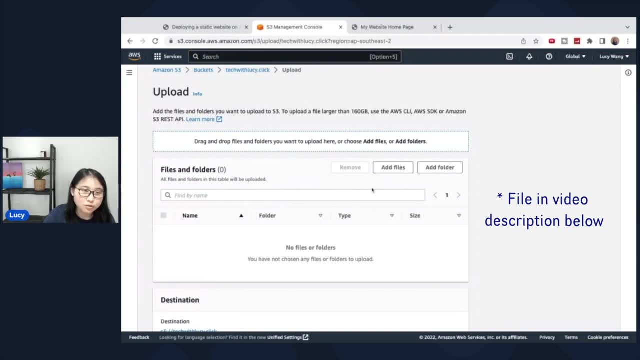 as a bucket. Click into your own bucket and select upload. So what we're going to do is we're going to upload our website and for this demo, I've decided to keep it very simple and just have a single page as the website. So I'm going to upload the content on my website, which is this: 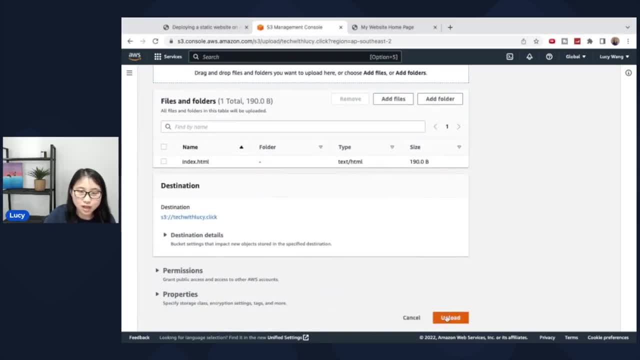 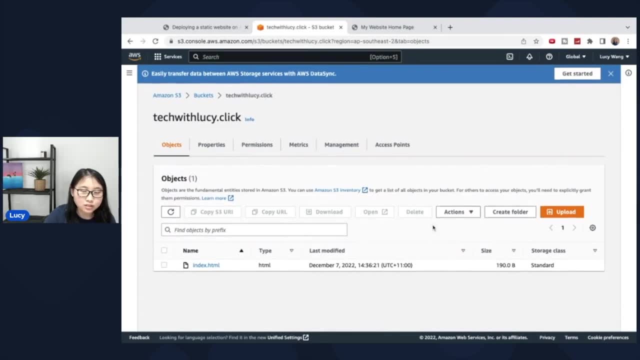 indexhtml file, Select upload and the page has been uploaded. What we're going to do is make sure that this bucket is enabled for static website hosting and making sure that it has the right permissions for users to access it. So, if you click on properties, scroll down all the way to. 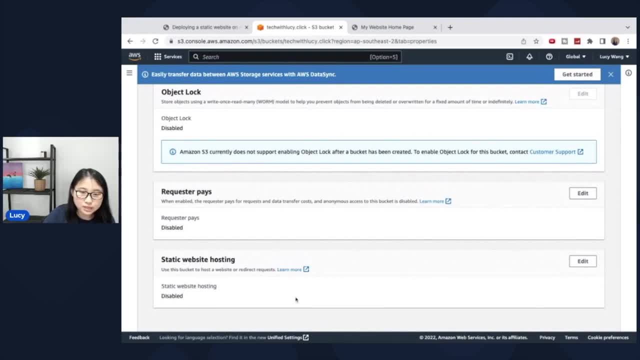 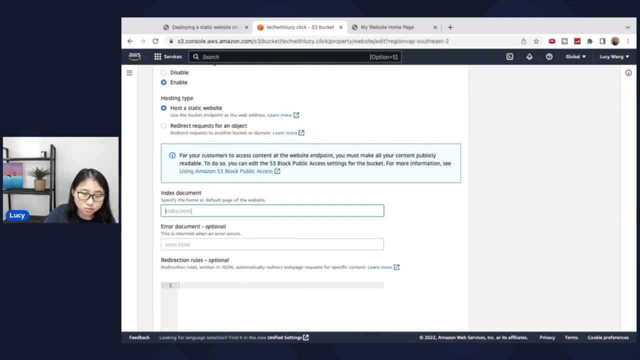 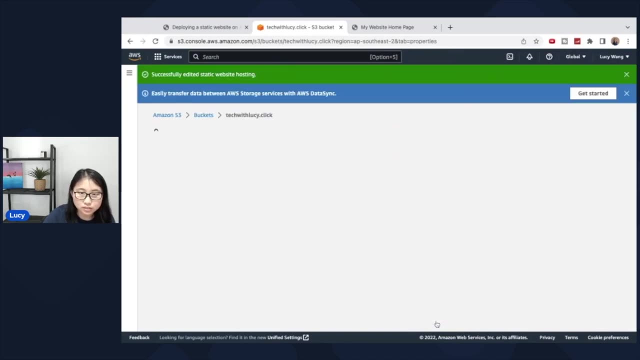 the bottom to static website hosting, You can see, by default it's disabled, but what we're going to do is enable it and at the index document- section type in the index document, in my case indexhtml- Click save changes. And another thing we need to do is on permissions, we need to attach a bucket policy. 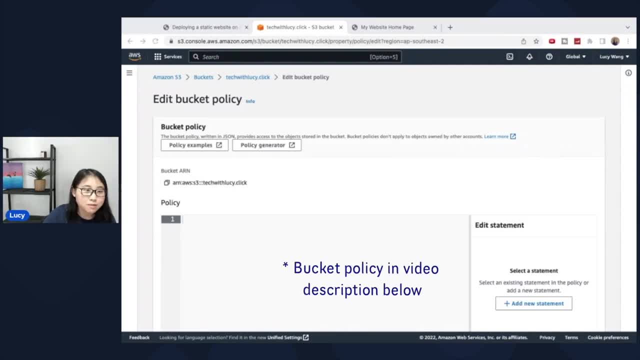 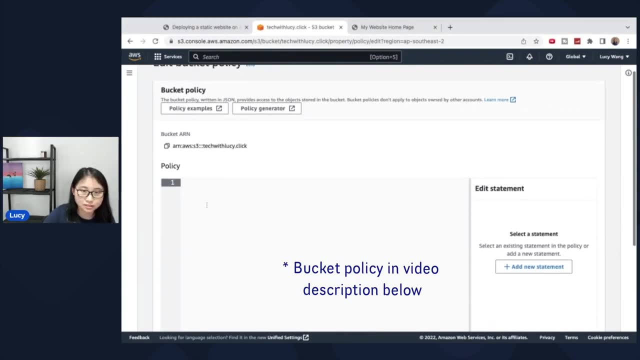 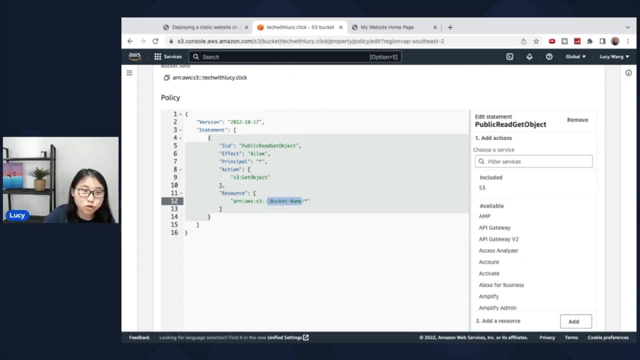 So click edit and put in a bucket policy. I'll provide this bucket policy in the details below so you can copy and paste this in Here. you can see that there is the bucket name, but you would have to put in your own bucket name. So I'm going to type in: 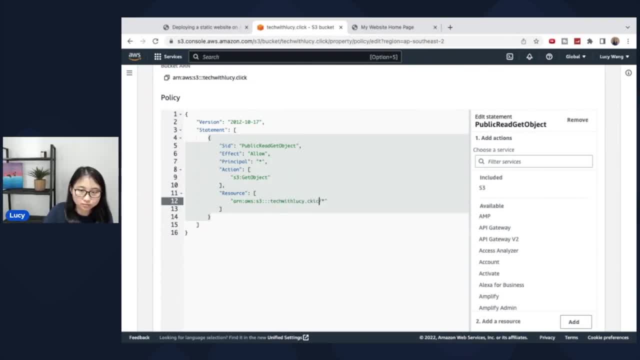 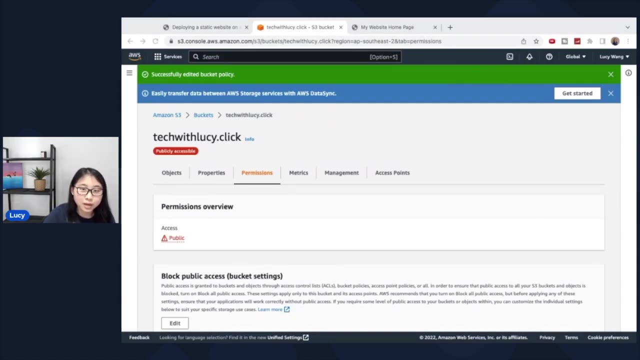 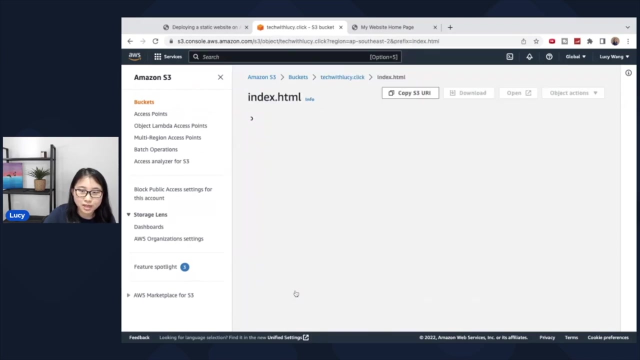 heckwithlucyclick. So this policy is only a template, so you'll need to provide your own bucket name in order for this policy to work. So click save changes and we've now configured the bucket to have the sample website publicly accessible for viewers. So once we go into this website, if you click on open, you'll see. 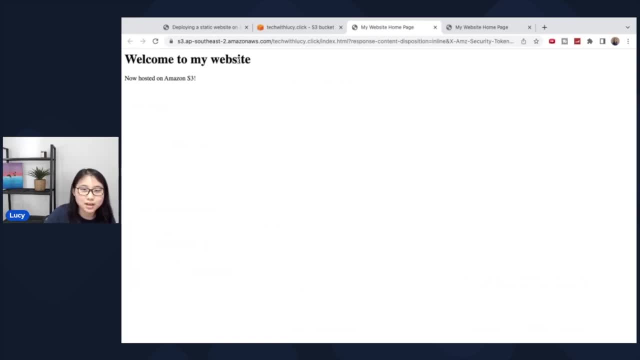 the welcome message. And you see, you know, welcome to my website, now hosted on amazon s3.. So what you've done at this point is you hosted the website on amazon s3 but, as you can see here on the url, it's not your custom url, this is a amazon provider url.